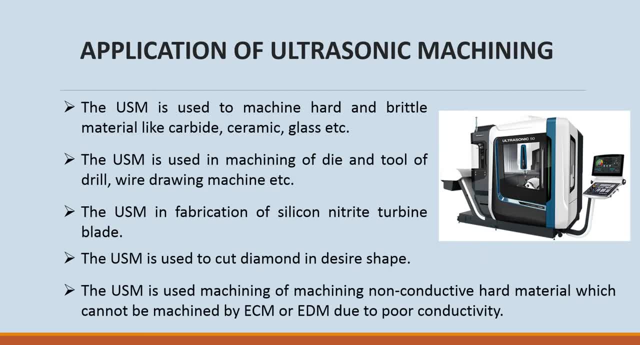 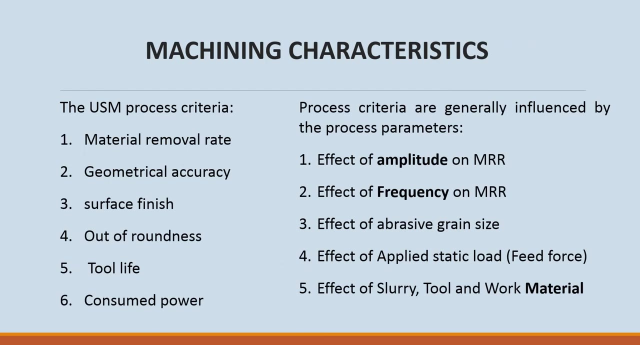 the figure. Ultrasonic machining has a lot of application for machining hard and brittle material for machining of die and tool of drill to fabricate silicon nitride, turbine and plate, and it is used to cut diamond in desired shape and so on. The main criteria for this process is material removal rate: geometrical. 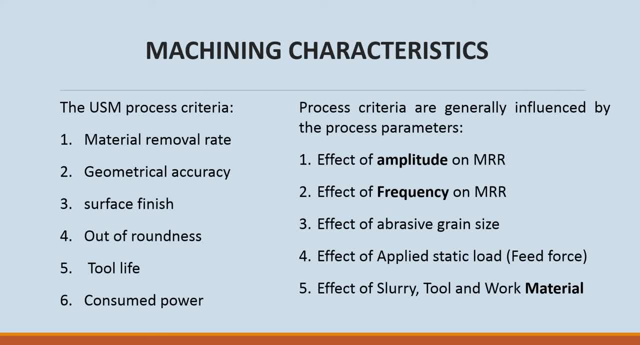 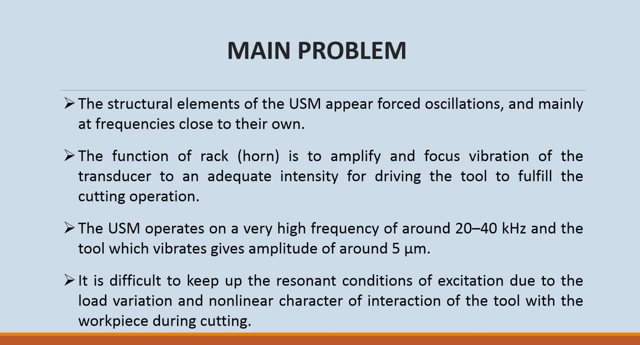 accuracy, surface finish, tool life, consume power and on this criteria affects the amplitude frequency, abrasive grain size, applied static load and material for tool work and slurry, And all of the subject of the machine- ultrasonic machine- is subject to the vibration. 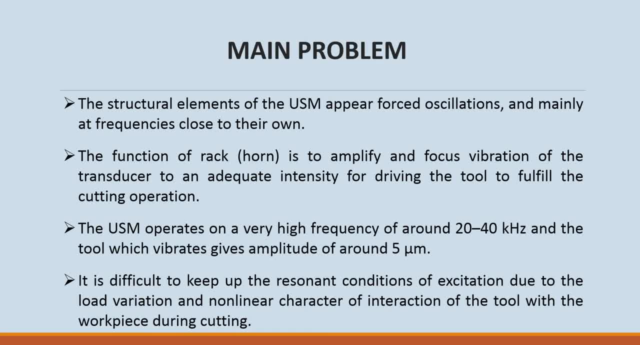 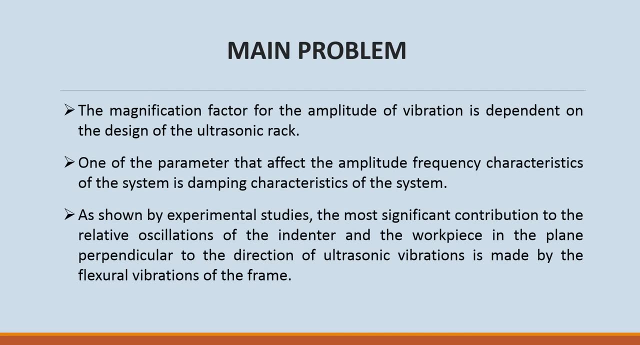 And this vibration is between 240 kilohertz and the tool. vibrates give the amplitude of around 5 micrometers And the magnification factor for the amplitude vibration is dependent on the design of the ultrasonic rack, and the damping characterist of the system is the main parameter that affects the 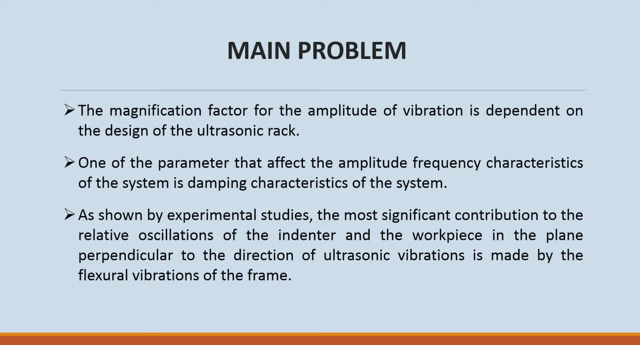 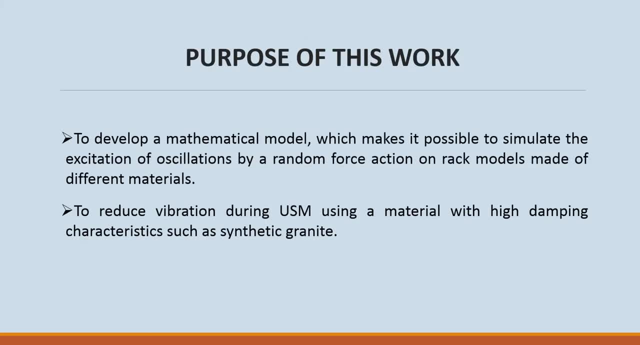 amplitude frequency of the system. actually So we. the purpose of our work is to develop a mathematical model which makes it possible to simulate the excited vibration of oscillation by a random force action on the rack. models made of different materials to reduce vibration during USM, using material with high damping capacity, such as synthetic. 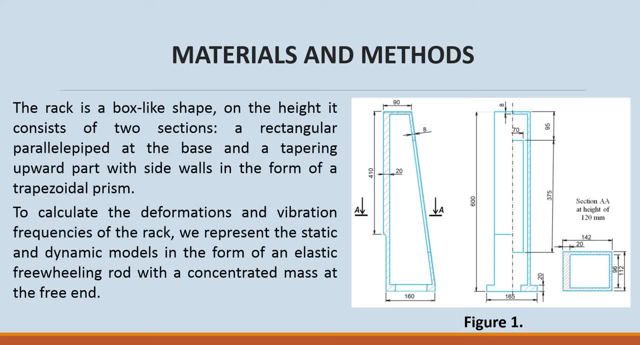 granite. So, as you can see from the figure, the rack is boxed like shape and on the height it consists of two sections. To calculate the deformation and vibration frequency of the rack, we represent the static and dynamic models in the form of an elastic freewheeling rod with a concentrated mass. 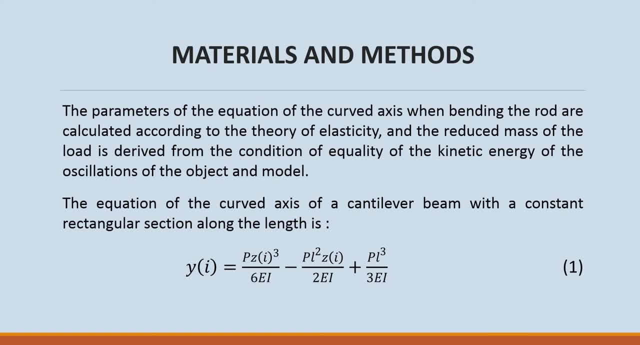 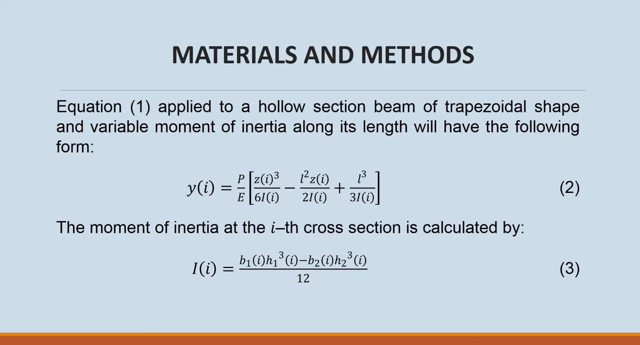 at the free end And we use the theory of elasticity. so we use the equation 1 to calculate the curved axis of a cantilever beam with a constant rectangular section And we apply this equation To hollow section beam of trapezoidal shape and variable moment of inertia along its length. 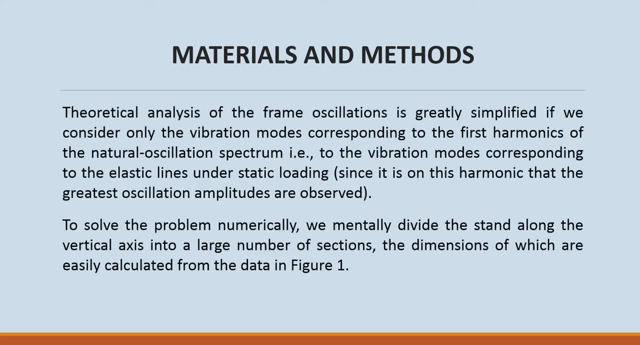 So I mean equation 2 and equation 3.. And theoretical analysis of the frame oscillation is greatly simplified if we consider only the vibration modes corresponding to the first harmonics of the natural oscillation spectrum. So Since it is not, it is on this harmonic that the greatest oscillation fields are observed. 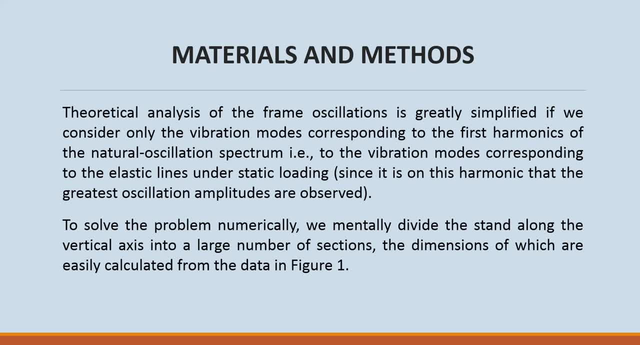 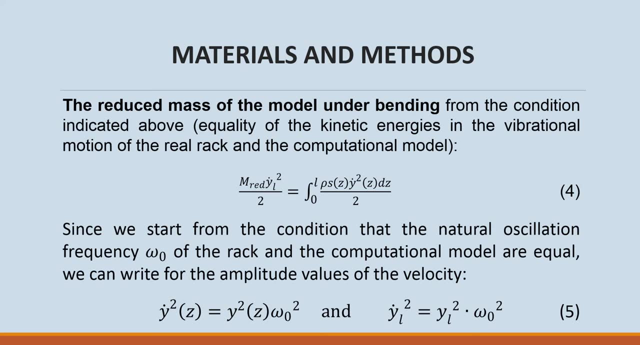 To solve the problem numerically, we mentally divide the stand along the vertical axis into a large number of sections, the dimensions of which are easily calculated from the data in figure 1.. So we achieve the reduced mass of model under bending. and since we start from the condition, 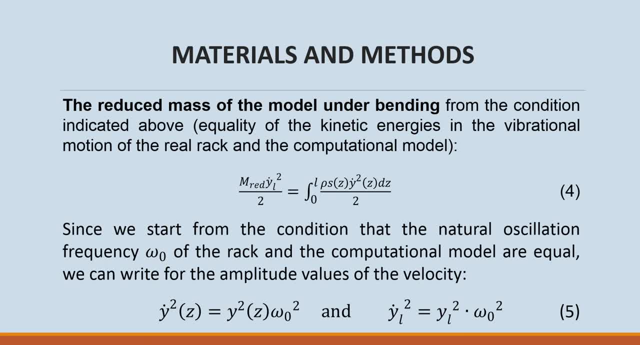 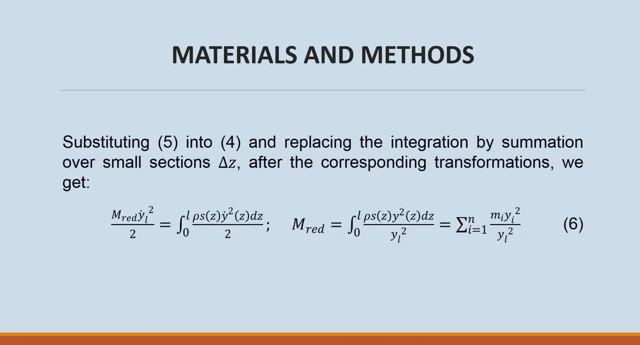 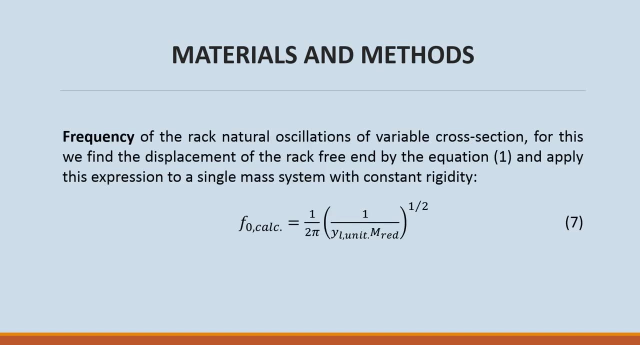 that the natural oscillation frequency of the rack and the computational model are equal. so we can write, for the amplitude values of the velocity, the equation 5.. We substitute the equation 5 to 4 and we get the equation 6.. And at the end we get the frequency of the rack. national oscillation of variable cross. 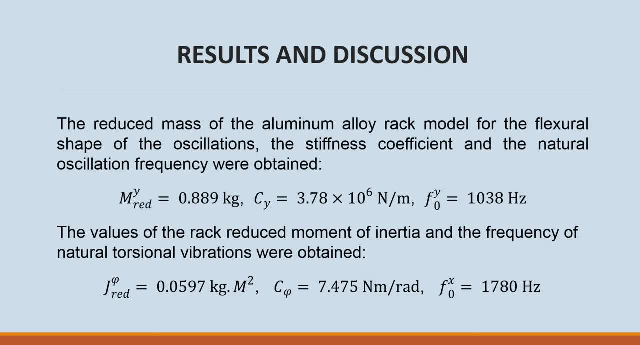 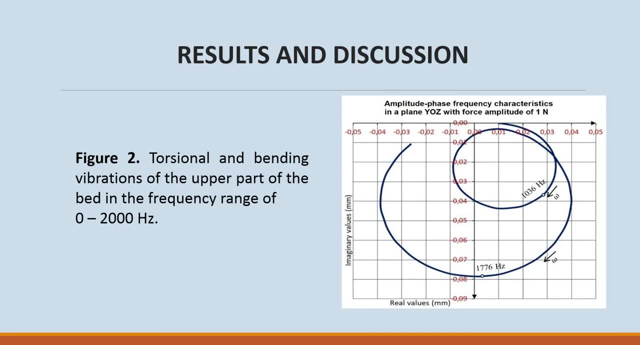 section. As a result, we calculate this equation for our case And we get the result. This is the end, Thank you. In high speed, the trouser bending vibration of the upper part of the break in theroom. frequency range of two is 0 to 2000.. 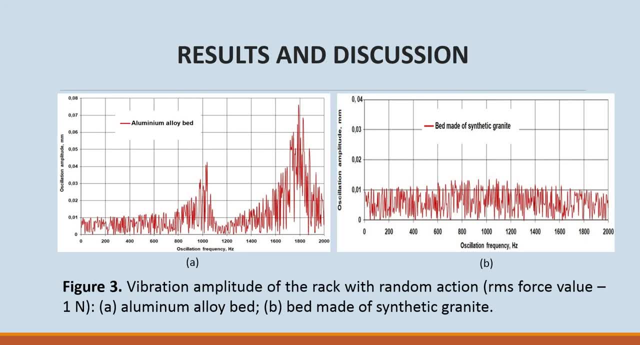 And as you can see in this, this slide compares the vibration amplitude of the rack for two different bits made of different materials. So, as you Can see, the bedfron made of synthetic granite has less Melissa amplitude. It means that it has better down in capacity. 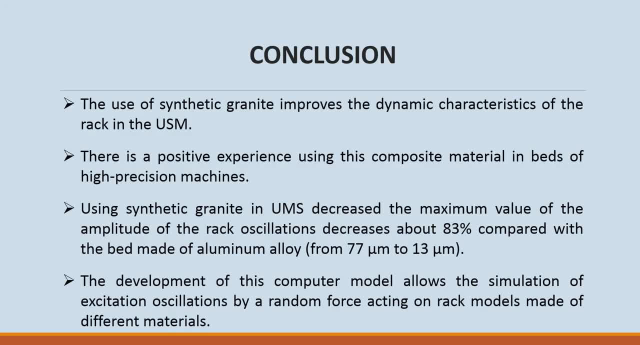 So what's the conclusions can say that the torsional bending pulses are distanced much from other waves. So this is the maximum. synthetic granite has decreased the vibration amplitude about 83% from 77 micrometer to 13 micrometer, and the development of this computer model 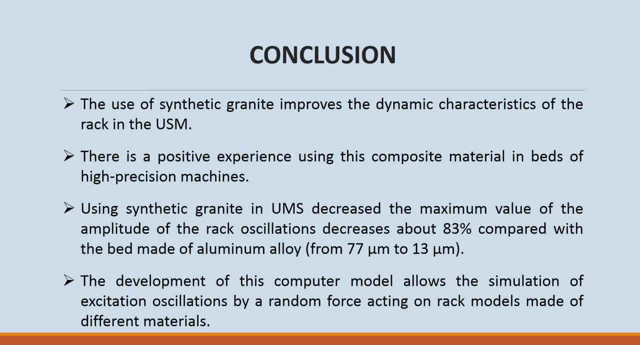 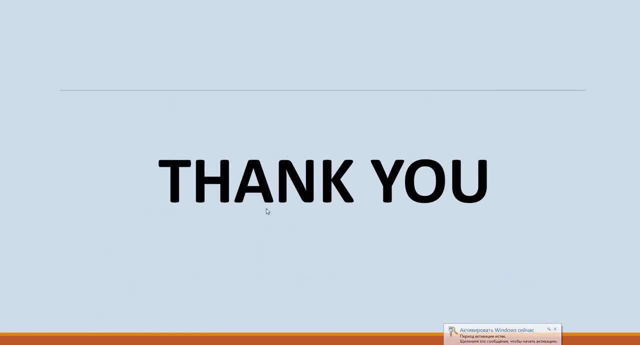 allows the simulation of the excitation oscillation by a random force acting on rag models made of different materials. thank you for listening.